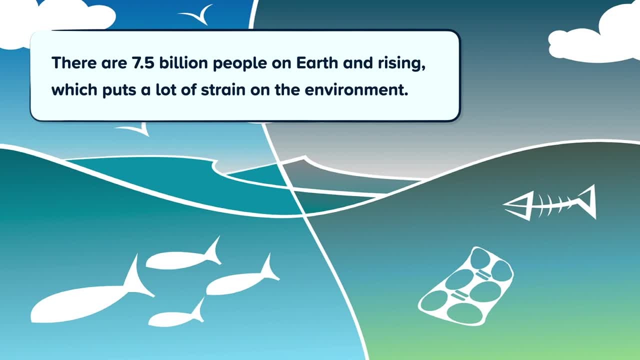 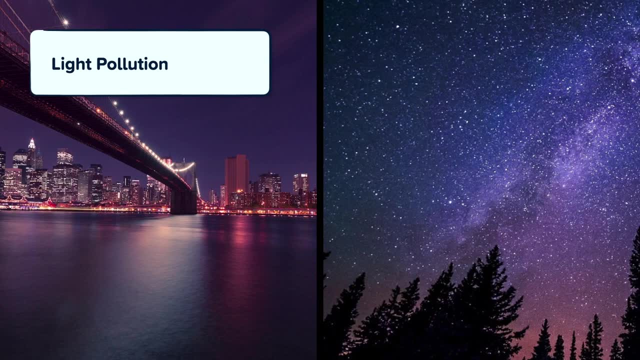 Now let's have a look at some specific ways humans impact the environment around them. Light pollution: Since life began, it has relied on the production of light pollution. Since life began, it has relied on the production of light pollution. Light pollution is a predictable cycle of night and day. It affects all sorts of behaviours from 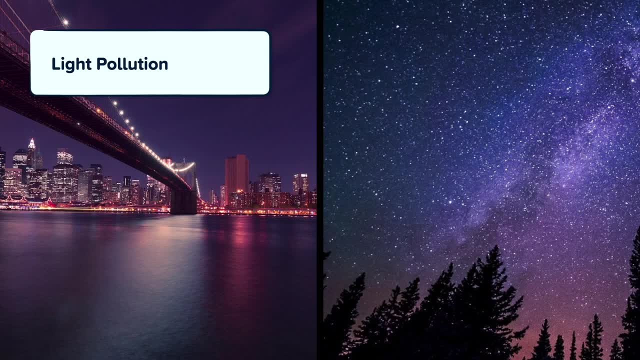 reproduction to sleep, even in humans. Artificial light at night has deadly effects on many animals. For example, predators often use light to hunt, but prey species will use darkness to hide. Also, baby sea turtles find the ocean by looking for bright light on the horizon and bright city. 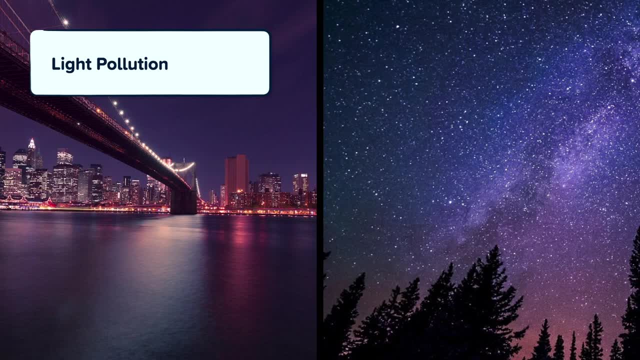 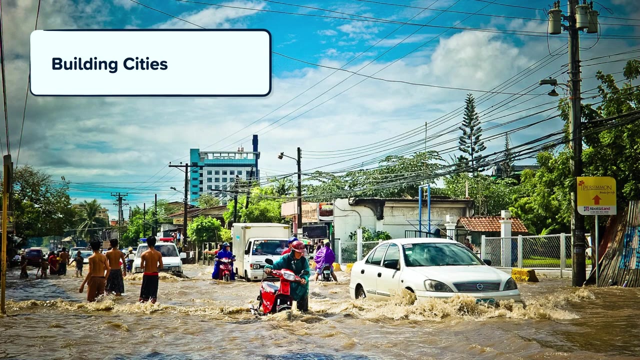 lights confuse them, so they go the wrong way, head inland instead of out to sea. Having very bright cities affects the way animals behave and this affects the ecosystem. Building cities and towns removes land for wild animals and plants to grow. Cities also have far fewer trees and plants and a lot more impermeable surfaces. 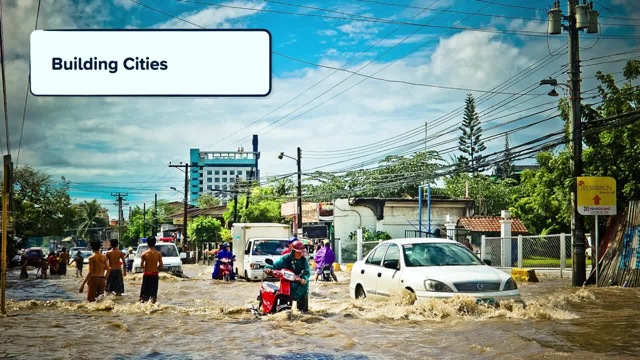 Impermeable means that fluid cannot pass through it. States of matter that can flow, like liquids and gases, are fluids, so impermeable surfaces don't let any liquids or gases move through them. So this means that water doesn't drain away as efficiently in cities and towns and it can cause flooding. 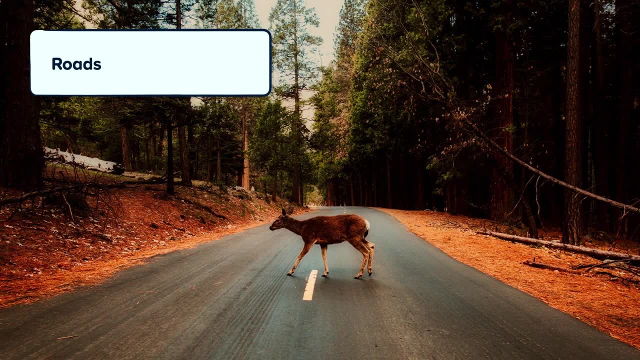 Roads directly harm wildlife. when an animal is hit by a vehicle, Roads can also affect animals behaviour. Some animals are attracted to roads and lights, and some try to stay as far away as possible from roads. This changes the species found in different areas. Roads also divide up habitats and can turn what was one large population into two smaller ones. 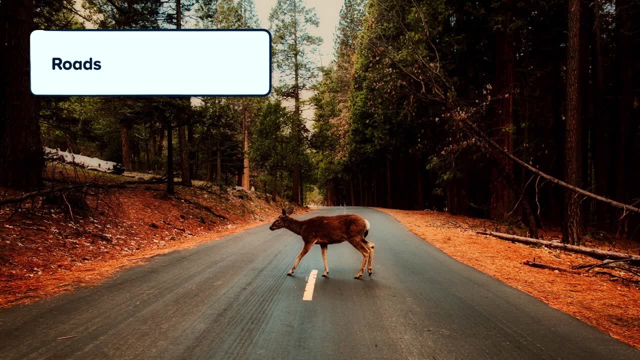 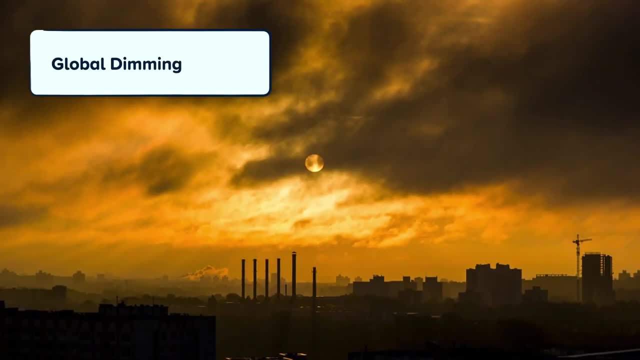 One on either side of the road that divides their habitat. Roads themselves also take up space and habitat is lost to build them. Global dimming. Global dimming reduces the amount of sunlight that reaches the earth's surface. It is caused by particles in the atmosphere that come mostly from 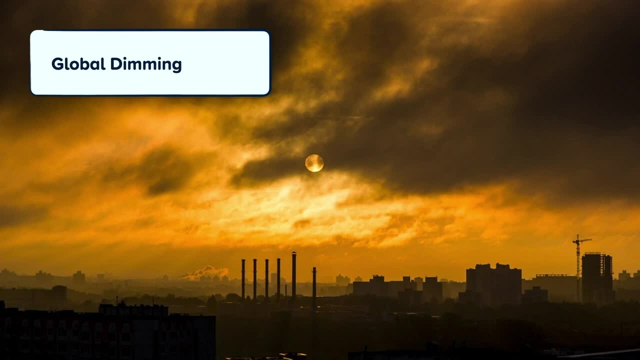 burning fossil fuels, There has been an average drop of 22% of the sunlight reaching the earth's surface, which is a big risk to ecosystems. Remember that all life depends on photosynthesis carried out by producers, and photosynthesis depends on light. Global dimming also disrupts the water cycle. 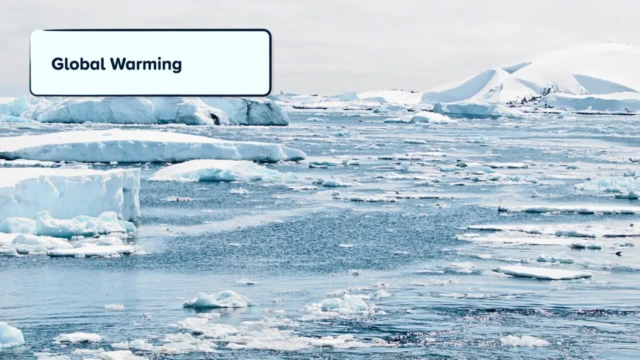 as evaporation is slowed down, Global warming, The earth's temperature has increased by about 1 degrees celsius since 1880.. Currently, the temperature is rising about 0.2 degrees celsius every 10 years. This doesn't sound like a lot, but it has a very big impact on weather patterns. 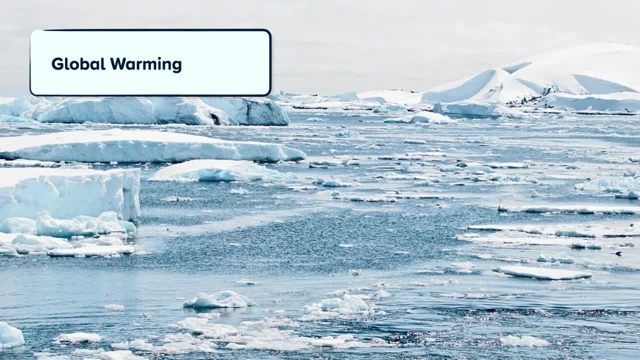 sea level and temperature of a habitat. It's important to note that the temperature rise is an average from across the globe. Some areas will become colder or get more rain as a result of an increase in average temperature. Extreme weather patterns are also a symptom of changes. 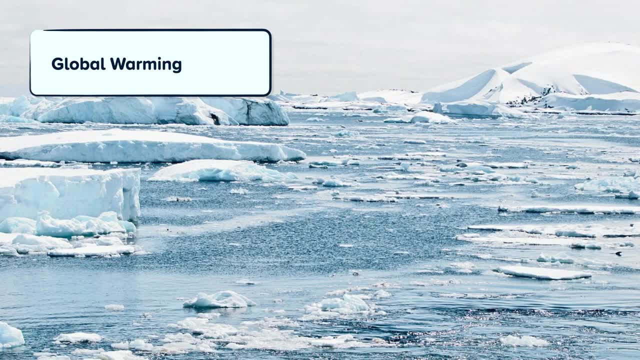 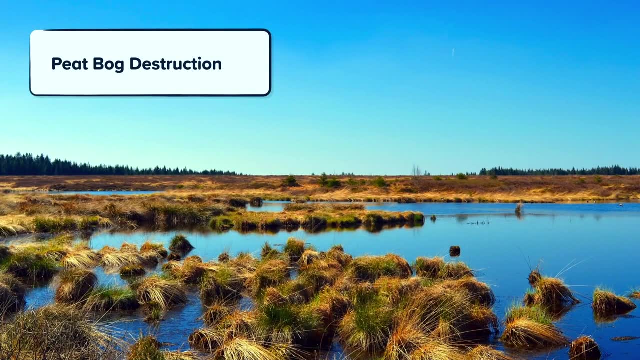 to the global temperature, Changing habitats forces species to move to new areas or die, which disrupts the food chains. Peat bog destruction. Not many people have heard of peat bogs, but they are incredibly important ecosystems. Peat bogs are wetlands where dead. 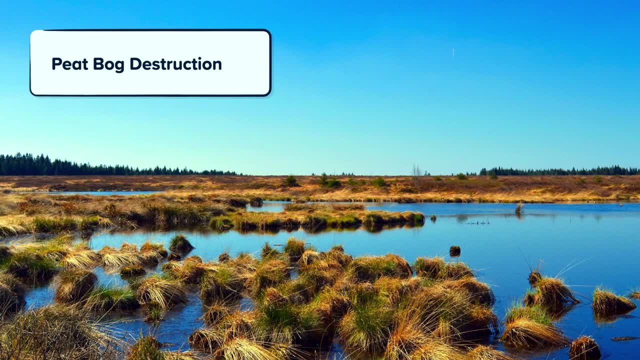 plants have built up to make thick layers. Oxygen doesn't get to the lower layers and over thousands of years peat is formed. Peat is important to humans because it's very rich in nutrients and can be added to soil we grow plants in. It can also be dried and burned as a 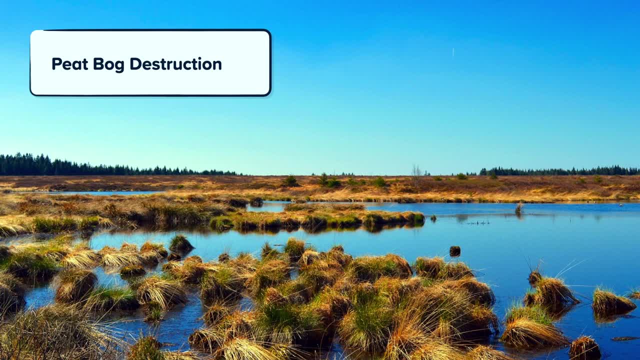 fuel. Humans will also drain these wetlands to build houses and farms. Peat bogs are very important habitats as they support a lot of different species and they lower flood risks. They also have a lot of carbon locked away in them which can be released. 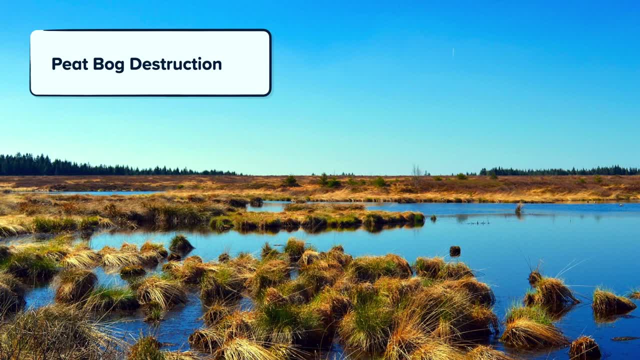 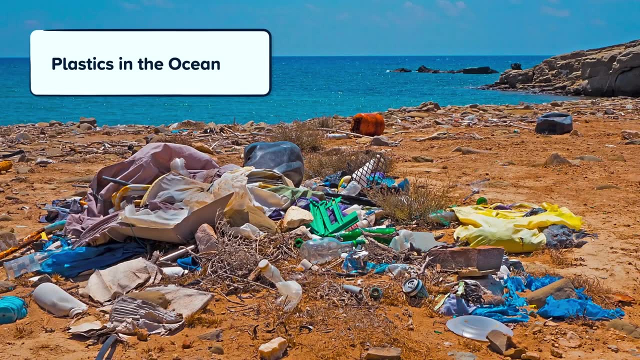 into the atmosphere as carbon dioxide when the peat is burned. Carbon dioxide is one of the greenhouse gases. Plastics in the ocean. Plastic is a very useful product to humans, but it does not break down in the environment. Eight to twelve tons of plastic finds its way into the oceans each 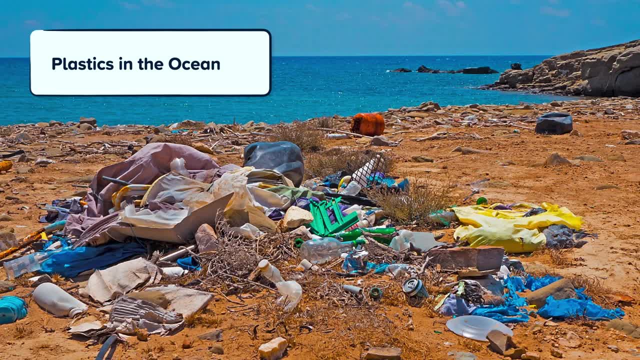 year, and this can harm all levels of the food chain. Many marine animals consume plastic, thinking it is food. This causes problems with growth and reproduction and even death. Plastics also carry pollutants that disrupt the way the body works. These can enter the food chain and be passed along. 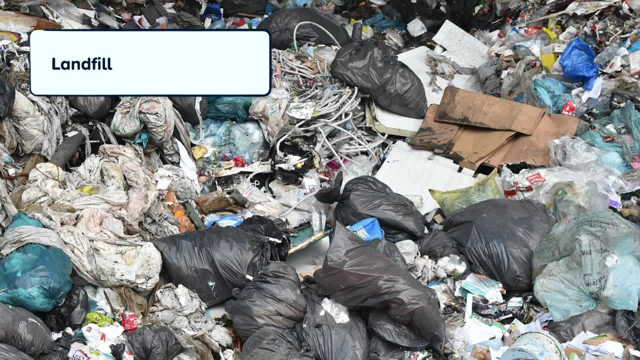 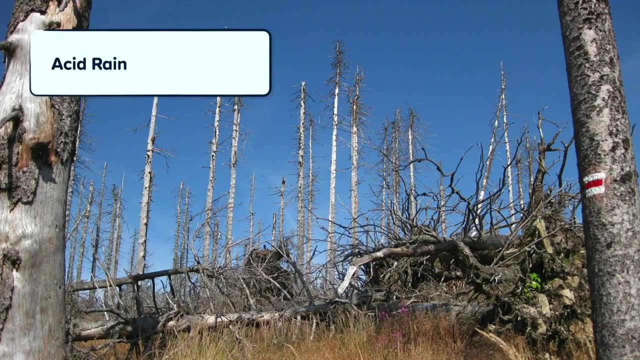 Landfill. Humans produce a lot of waste products and often bury them in landfills. This removes habitat for plants to grow and animals to eat. Landfills also release pollutants into the air, soil and nearby water- Acid rain. When some fuels are burned, they release a gas called sulfur dioxide. 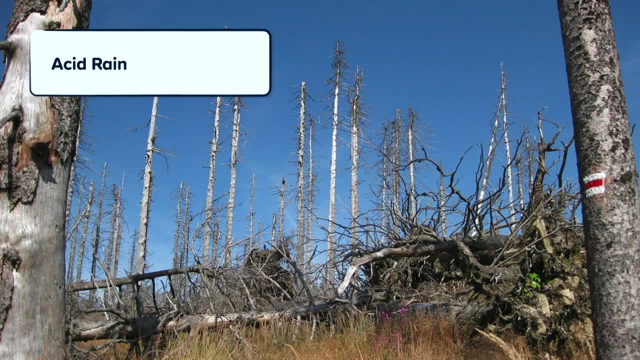 Also when air gets very hot, such as inside a car engine. nitrogen and oxygen in the air can react together to make nitrogen oxides. Both sulfur dioxide and nitrogen oxides dissolve in rain and make it acidic. Acid rain damages plants, soils, leaves and other elements of the environment. This causes a lot of damage to the 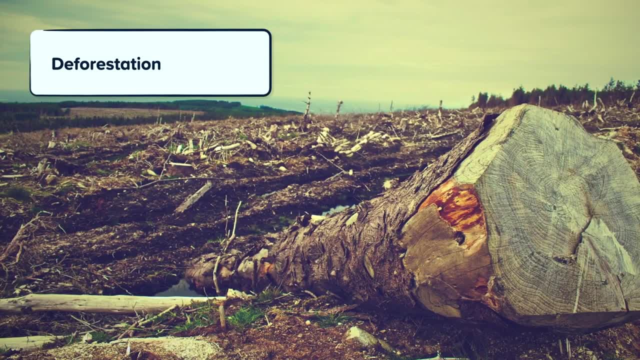 environment Deforestation. Deforestation removes trees and other plants from an area so that humans can use the wood and the land it was growing on for things like farming. This completely destroys whole ecosystems. The animals no longer have a place to live or things to eat, so they must move. 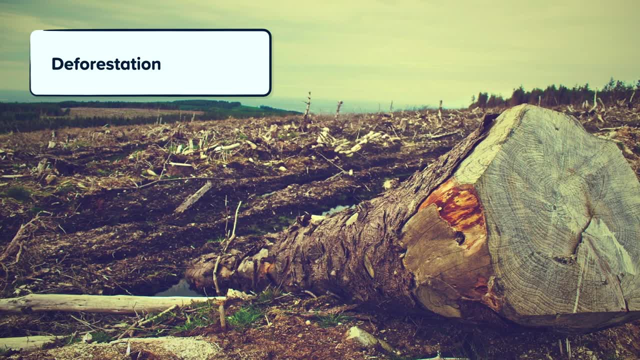 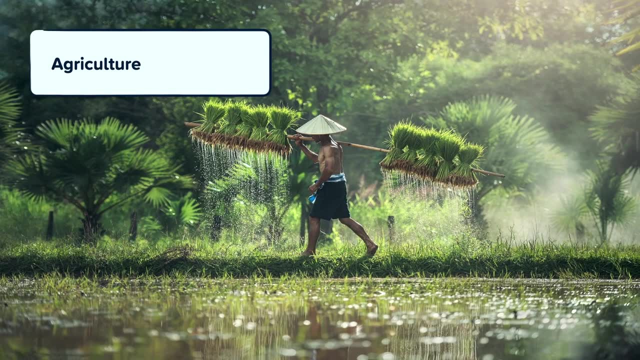 to a new area or they might die. If they move to a new area, this will disrupt the food chains of the organisms already living there. Agriculture- Agriculture Building farms- removes habitats, so wild plants and animals can no longer live there. Pesticides are chemicals that kill pests. Fertilizers provide nutrients for crops. 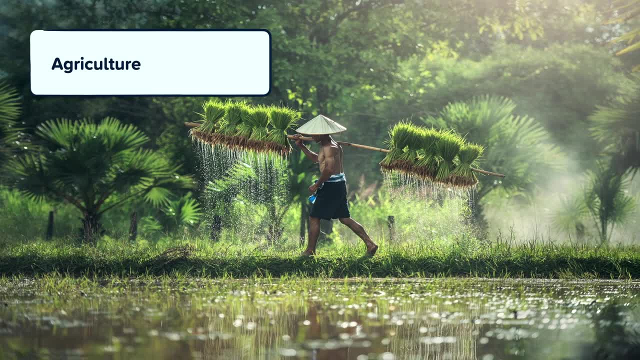 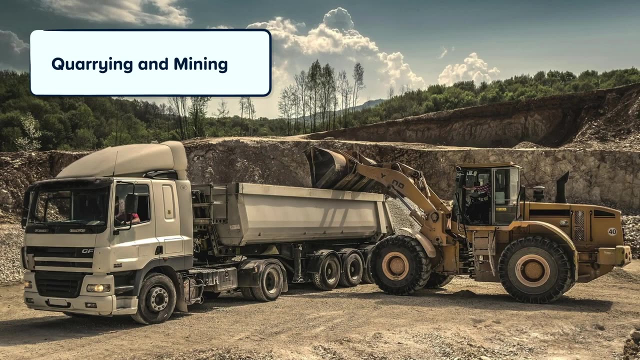 and herbicides kill plants that grow where we don't want them to grow. These chemicals find their way into the ecosystem very easily and damage it. For example, pesticides will kill beneficial insects as well as the pest species. Quarrying and mining: The materials that humans use, such as rocks and metals, are dug out of the ground in quarries and 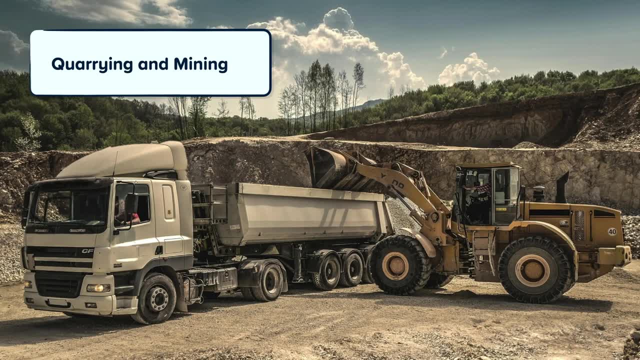 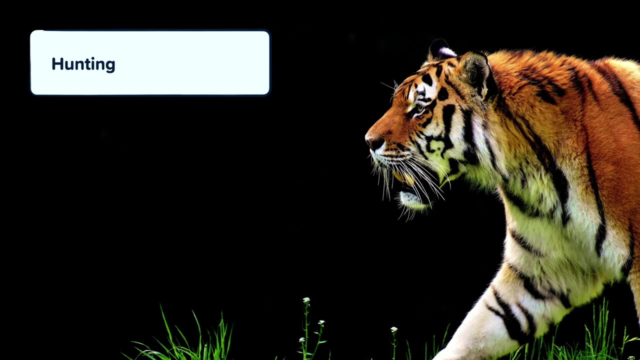 mines. This removes habitat for plants to grow and animals to live, just like with buildings, agriculture, deforestation and landfills. Quarrying and mining also produces pollution, with all the machinery and vehicles required for it. Hunting Wild animals are often killed by humans: 100 million sharks, 20,000 African elephants, the 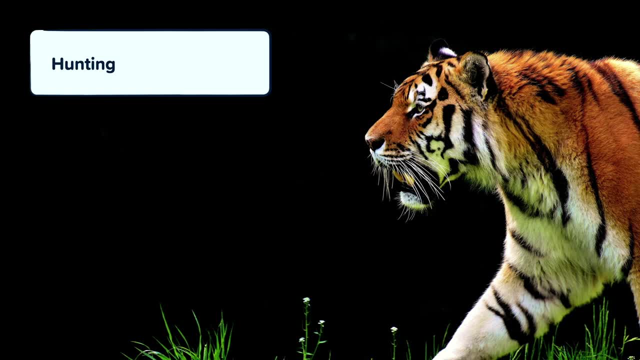 100 tigers are killed every single year. Sometimes people are hunting for food or for clothing, but a lot of the time the animals are hunted for sport. Many animals have already been hunted into extinction and many more endangered as a result of hunting. Nature is delicately balanced, so removing 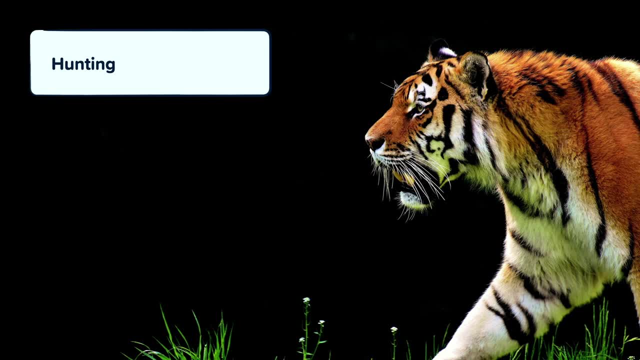 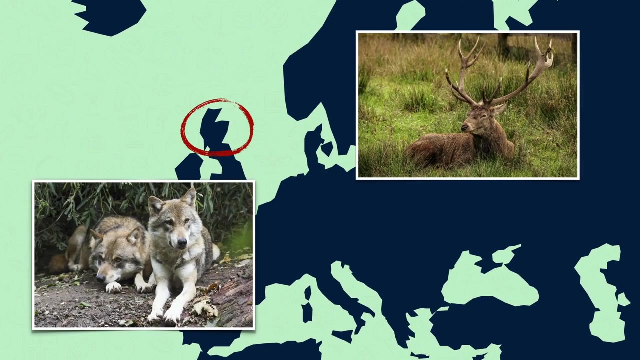 a species or reducing their number can have a big effect on food chains and therefore the ecosystem. Sometimes ecosystems become so out of balance that humans hunt a species, trying to stop the ecosystem from collapsing. For example, all the wolves in Scotland were killed by hunters and numbers of their prey animals increased rapidly. They ate loads of plants. 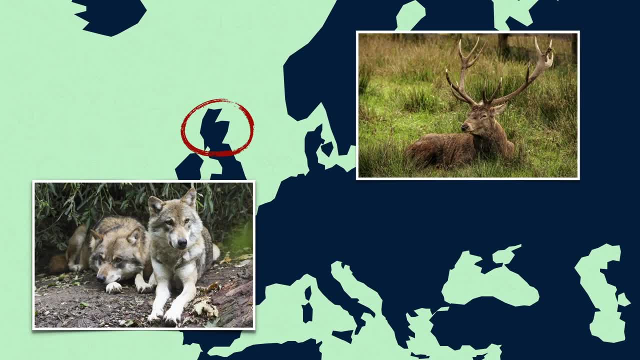 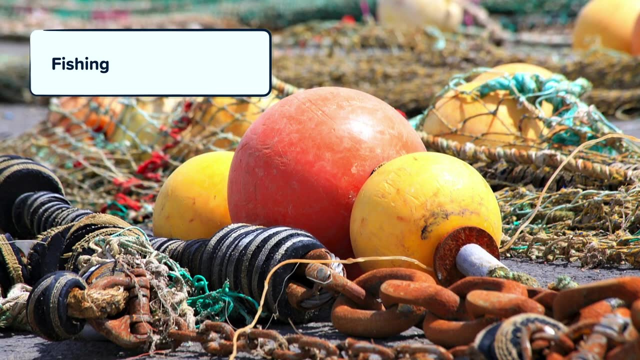 leaving whole areas. barren Humans now hunt just enough deer to keep the population in balance, but if the wolves had never been killed in the first place, the ecosystem would have remained in balance. Fishing Fish are a vital part of aquatic ecosystems. They are also an extremely 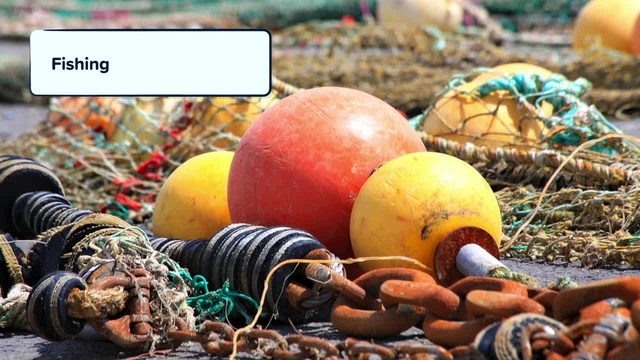 important food source for many people around the world. They are important for food chains and for nutrient cycling. They store a large amount of nutrients in their tissues that can go back into the environment when they die, Removing the fish for humans to eat in. very 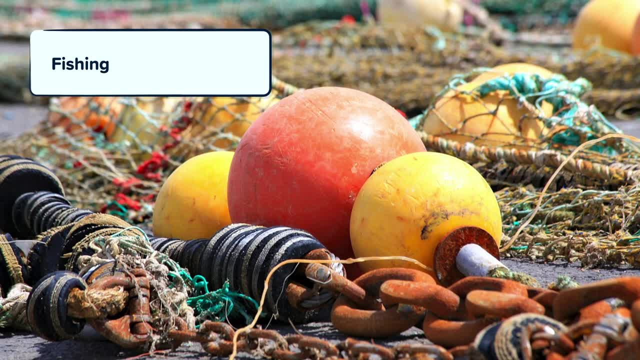 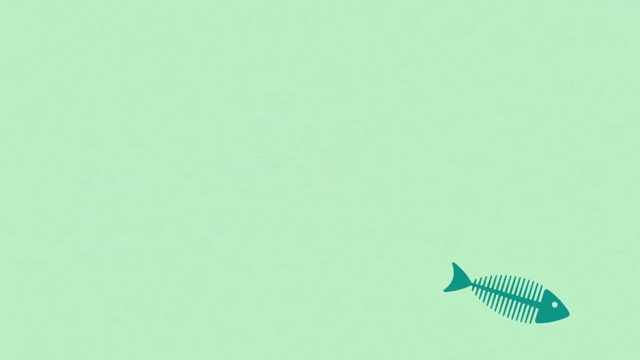 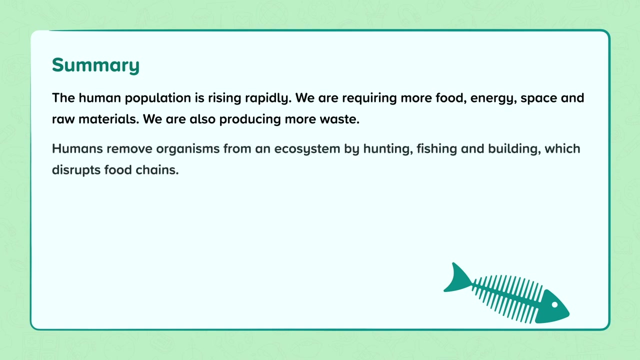 large numbers not only removes fish from the food chains, it also removes the nutrients that should have gone back into the ecosystem when the fish died. To summarise, The human population is rising rapidly. We are requiring more food, energy, space and raw materials. We are also producing more waste Humans remove. 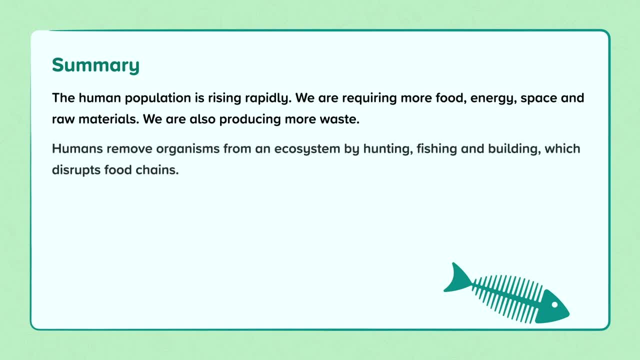 organisms from an ecosystem. by hunting, fishing and building, which disrupts the food chains, Humans change the landscape and use artificial lights, which changes the behaviour of some organisms. Pollutants have found their way into land, water and the air. These all affect the 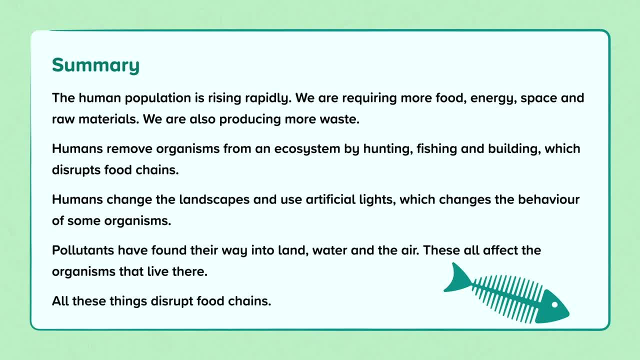 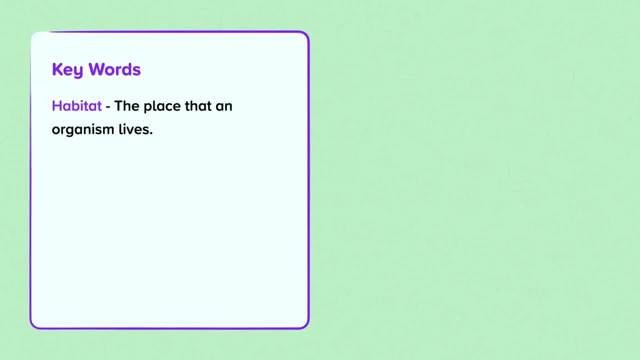 organisms that live there. All of these things disrupt food chains. Keywords: Habitat: The place an organism lives. Environment, The conditions surrounding an organism. Population: A group of the same species living in a habitat. Community. All the different types of organisms living in a habitat Ecosystem, A community of organisms. along with the physical